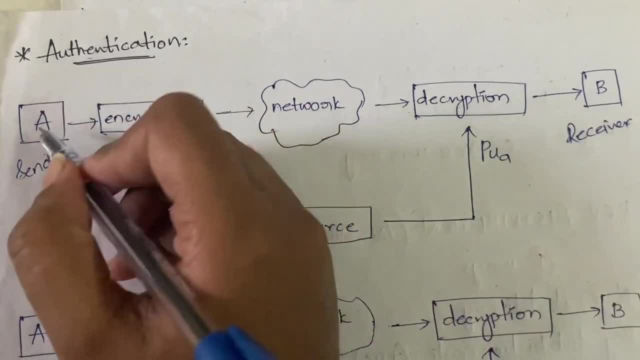 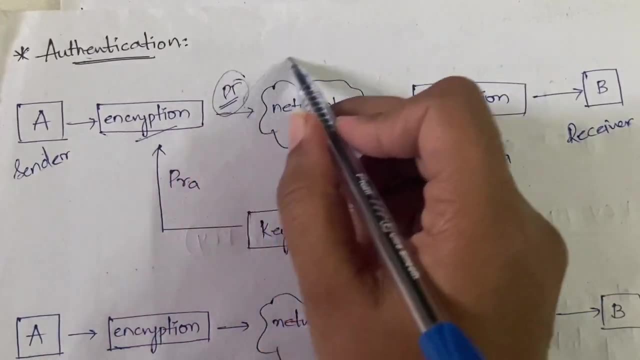 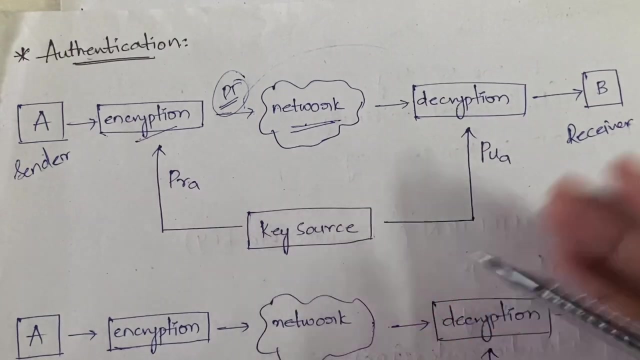 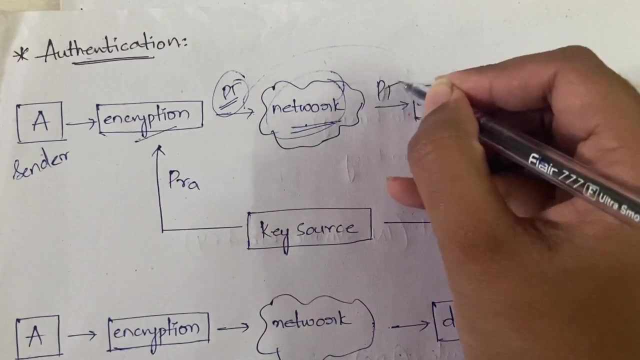 we have the sender and we have the receiver. So, first A, what A will do? it will encrypt the message, right, So it will encrypt the message and it will generate the plain text. This plain text will be carried over to the receiver and, through the network, It may be anything, It may be internet, it may be email or a message, whatever it is. So, with the help of network, it will be transferred to the other side. So, on reaching the other side, this plain text will be decrypted and it will be converted. Sorry here, sorry, sorry. I 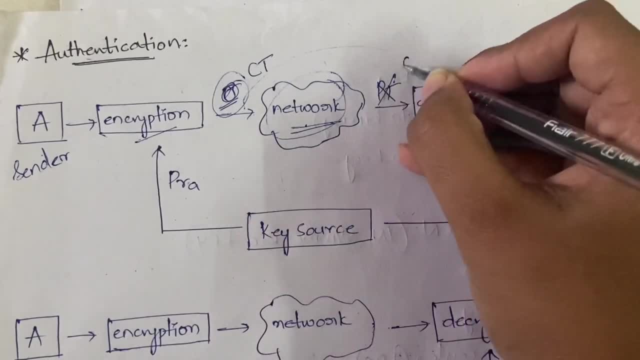 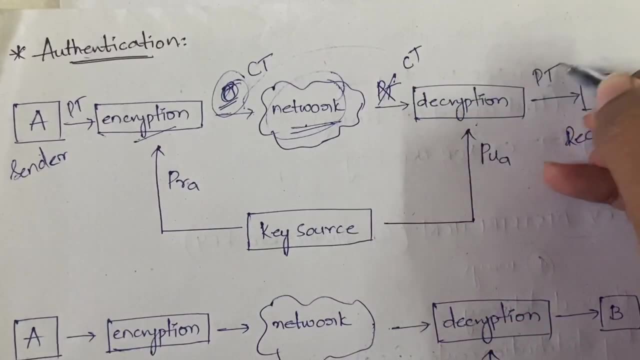 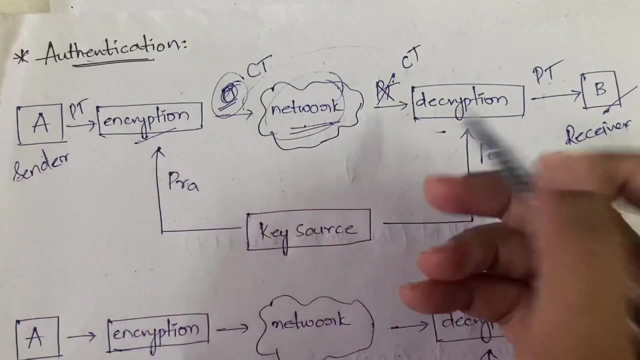 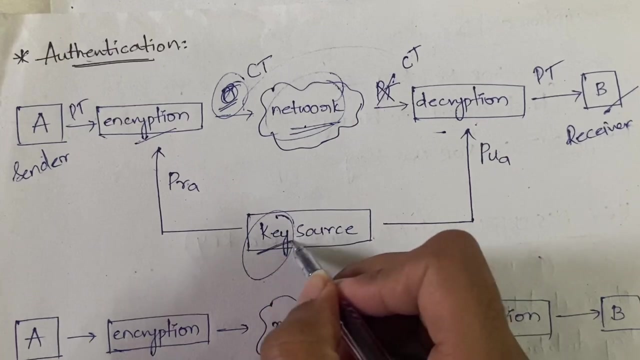 am really sorry. Here you get the ciphertext right Here. here it is the plain text. Plain text is converted into ciphertext and then the ciphertext is again decrypted and you get the plain text back. So the receiver will be getting the plain text back. So, in order to do both encryption and decryption process, what is the important thing that you need? You need the key, right. Right, You need key. So this key is provided by key source. So, ultimately, what is the main point here? 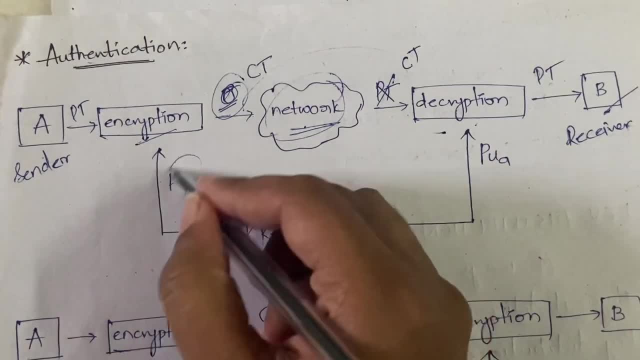 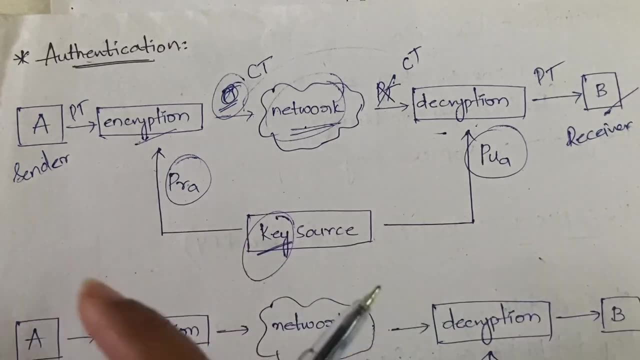 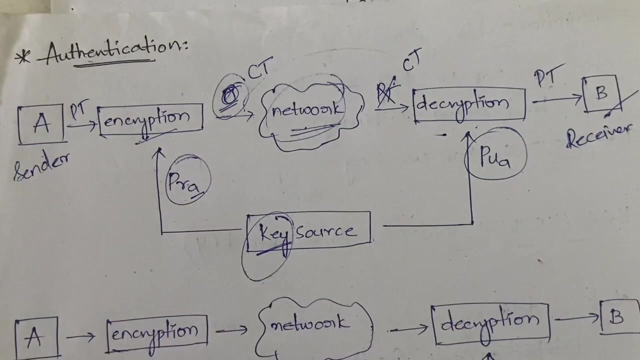 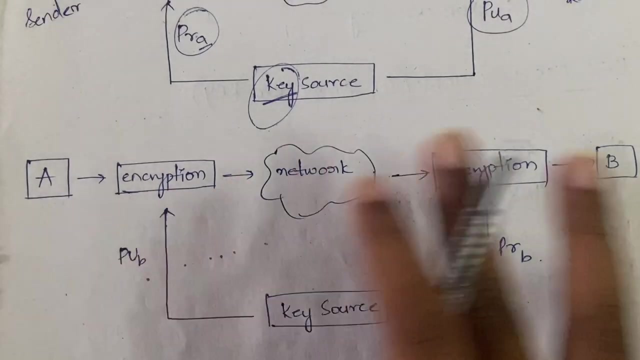 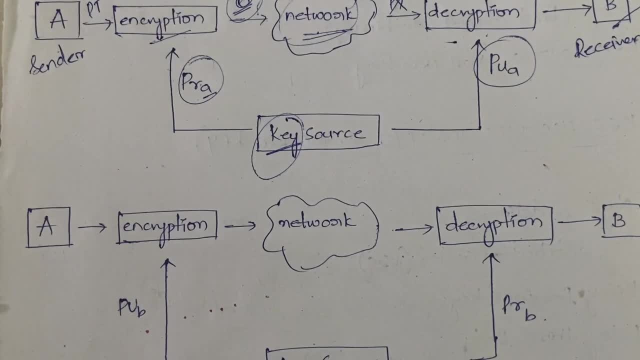 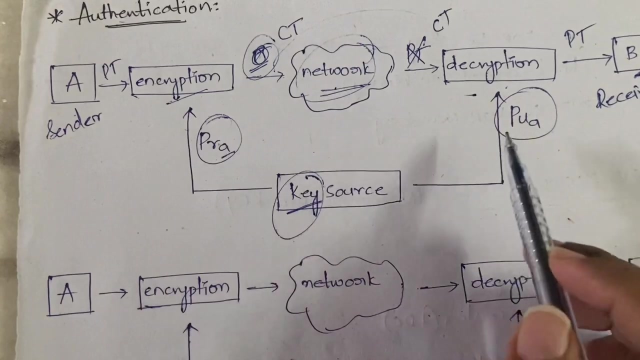 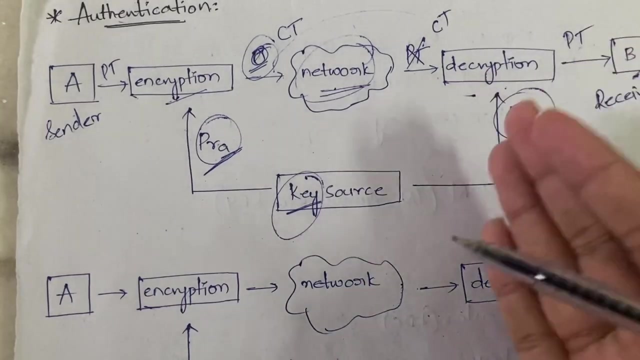 That is the difference. All right, So you will be sending two keys, two different keys, but those two different keys will be from same source, either from the sender or either from the receiver Got it? This is what authentication means, And if both the keys are from A, then A for A side you will be giving the private key and for the B side you will be giving the public key. That is, if both the keys are from A for its same side, for the same side, that is, for A you. 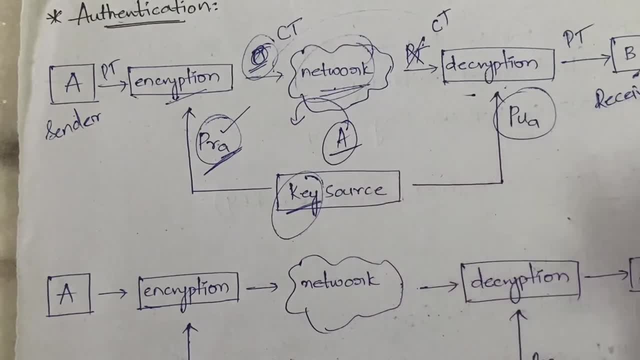 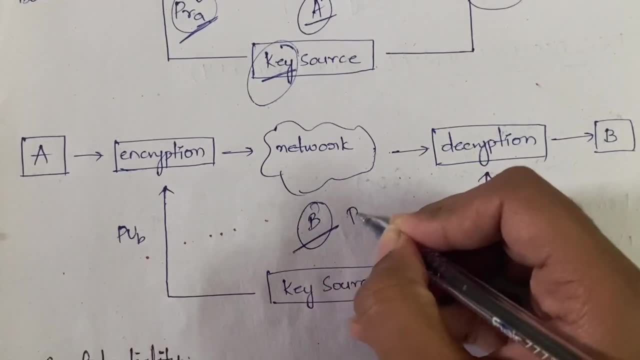 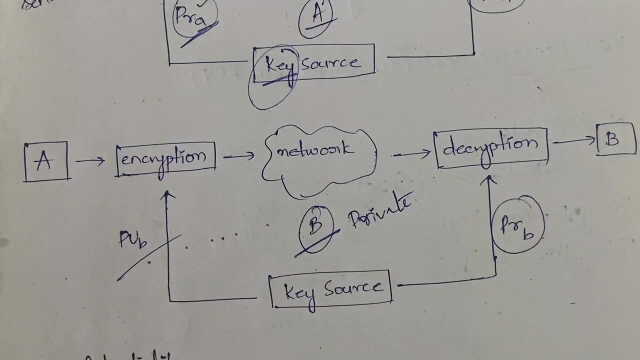 will be giving the private key. For B you will be giving the public key of A. Got it Now. here also, both keys are from which side? Both keys are from the side of B, right? So for B side you will be giving the private. So here private key of B and here it is the public key. So whichever source you are using, that source side will have the private key. the other will have the public key because its private key it cannot share with others- other people, right? This receiver cannot share his private. 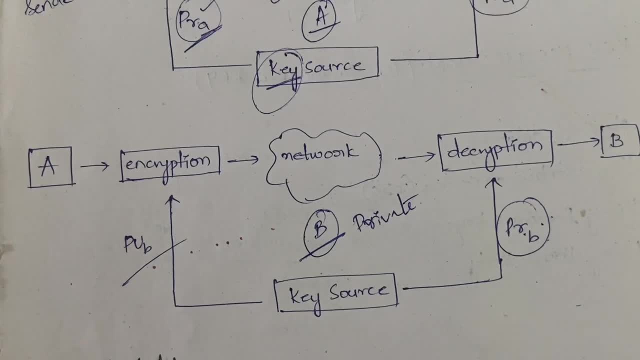 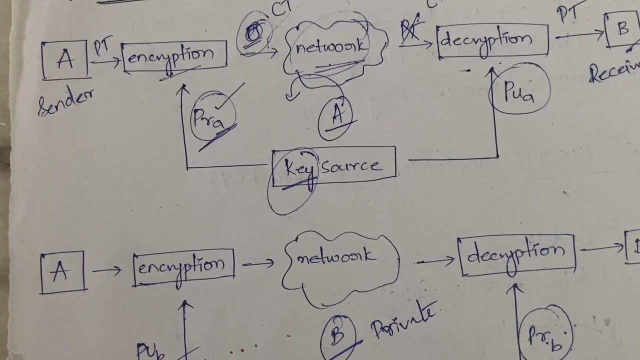 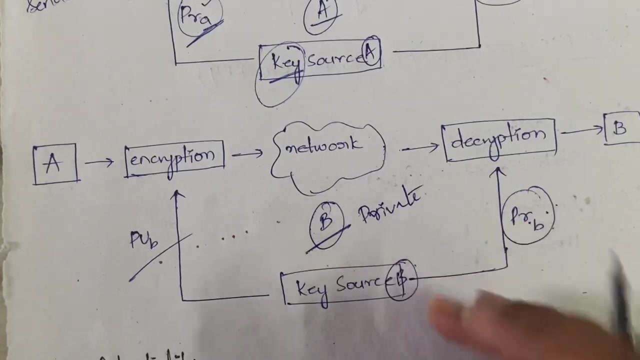 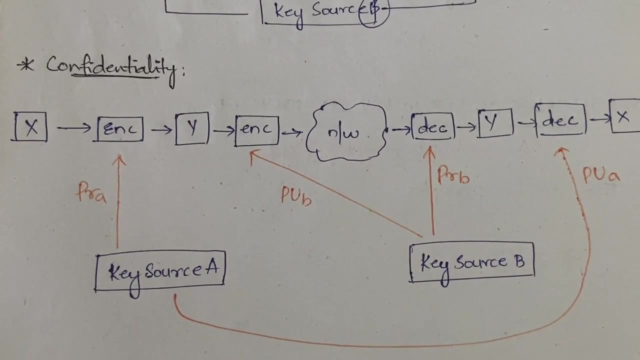 key with the sender, right? So this is all about the authentication. In authentication you will be using the. whatever keys you are using, two different keys will be from the same key source. Got it, Either from A or either from B. Got it? So this is about the authentication And the next thing we have is the confidentiality. This is going to be a bit complicated, but don't get confused. So first, X, X is encrypting the message and Y is generated. Again, Y is 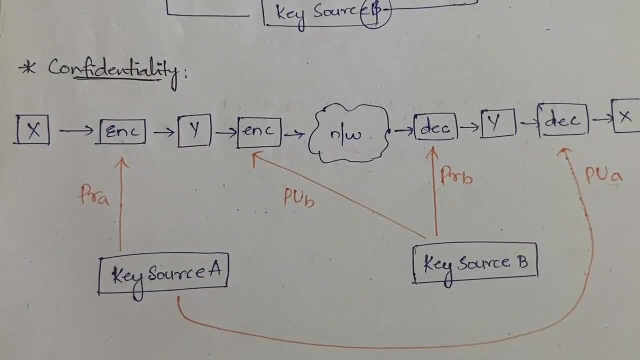 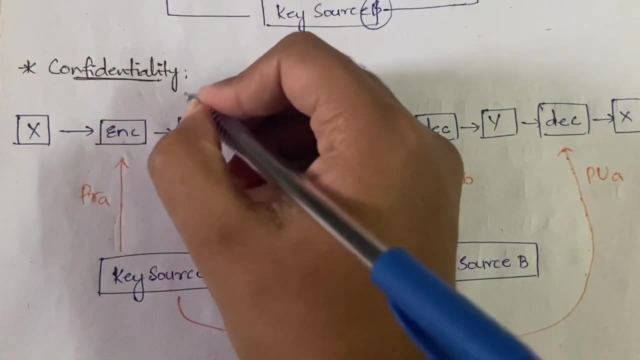 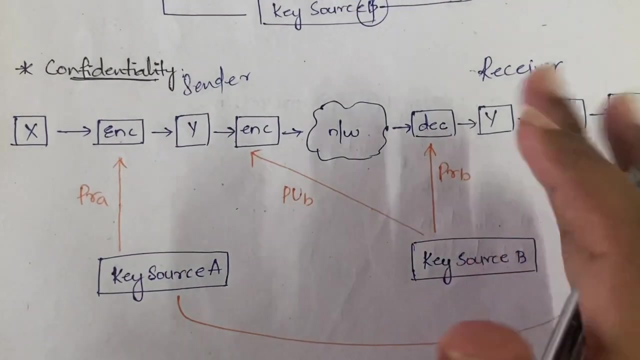 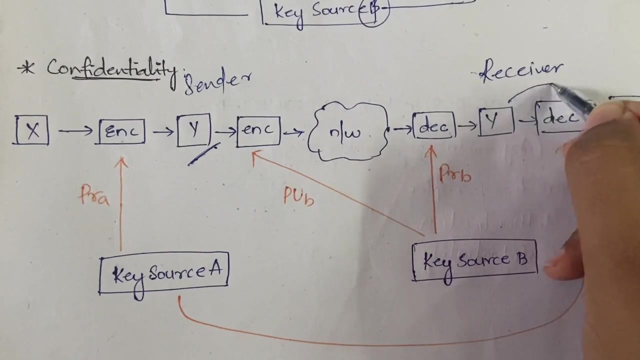 encrypted and again some ciphertext is generated. okay, So here we are doing two times encryption On reaching the receiver side. so this is sender side, as you know already, and this is the receiver side, right? So on reaching the receiver side, what happens? First decrypted, First what is decrypted, Y is decrypted right. So then again Y is decrypted again to get X right. This is how the process is going on. Now for the 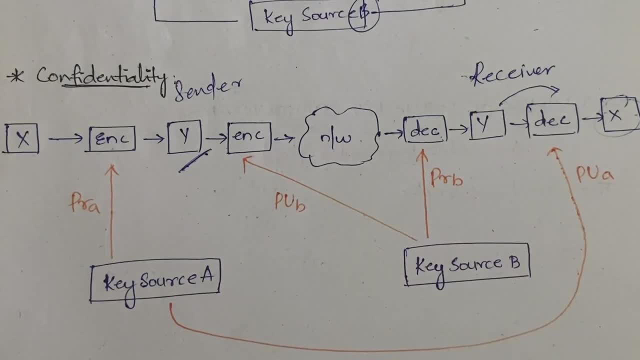 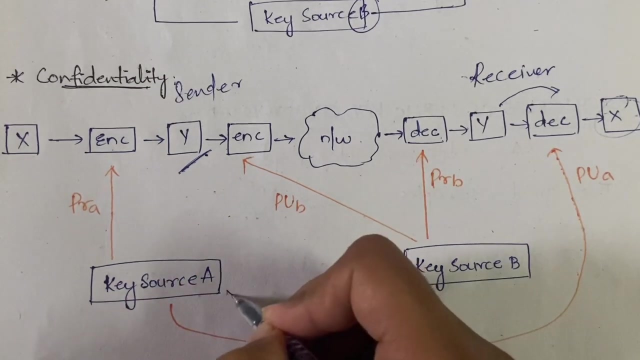 both these encryptions and decryptions key has to be provided right. So this key will be provided by two different sources, Whereas in authentication we have a single key source, But whereas in confidentiality we will have two different key sources. Got it? So this is the main difference between authentication and confidentiality, The two principles, authentication and confidentiality. Got it? So now let us see. So this key source of A is for X, Got it? And we are giving this key source of B for Y. So from